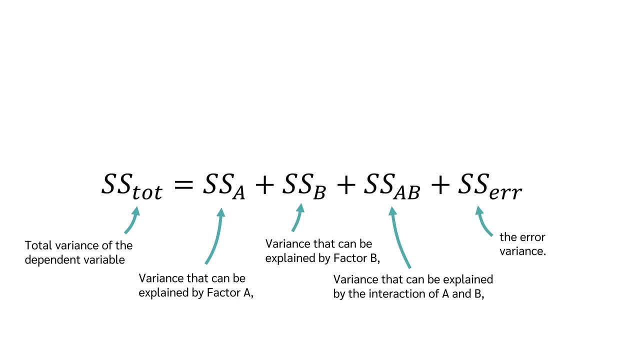 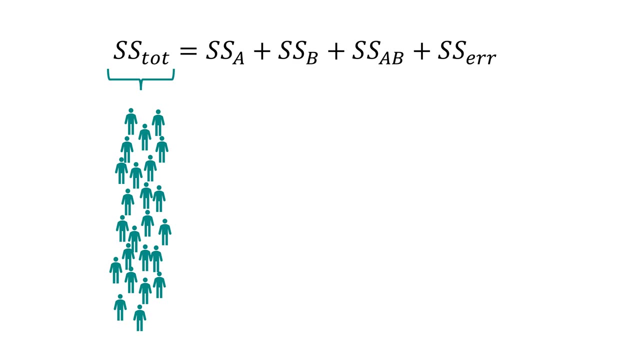 Actually, SS is not the variance but the sum of squares. We will discuss how to calculate the variance in this case in a moment. But how can I imagine that The dependent variable has some variance In our example? not everyone will have the same reduction in blood pressure. 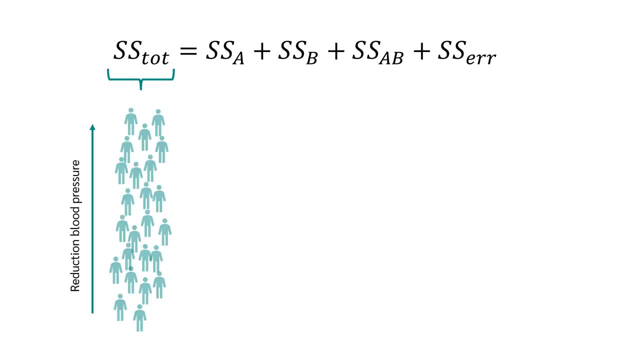 We now want to know if we can explain some of this variance by the variables: drug type, gender and their interaction. The part that we cannot explain by these three terms accumulates in the error. If the result looked like this, we would be able to explain almost all the variants by: 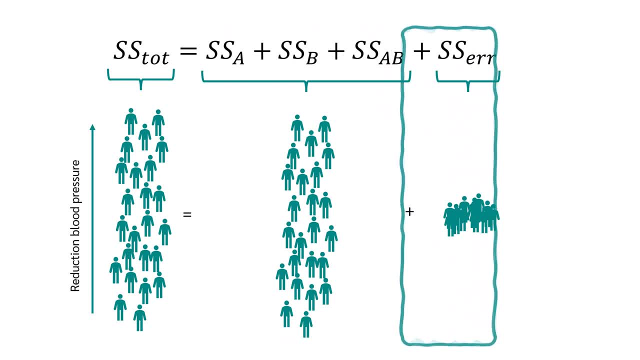 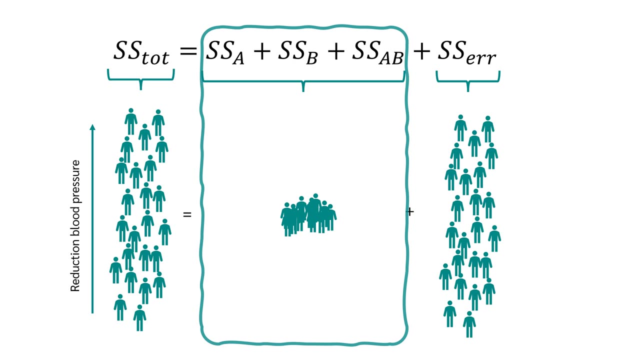 factors A and B and their interaction And we would only have a very small proportion. that could not be explained. In this case it would be the other way around: Drug type, gender and the interaction almost have no effect on the reduction in blood pressure. 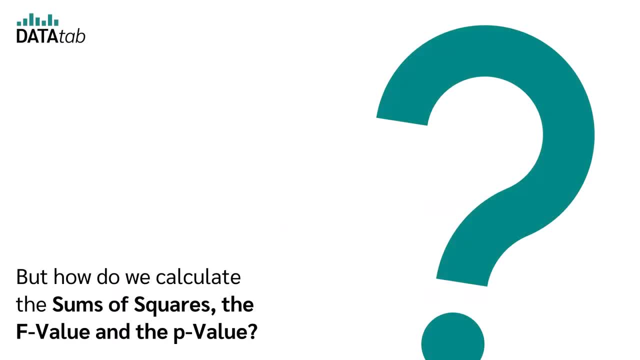 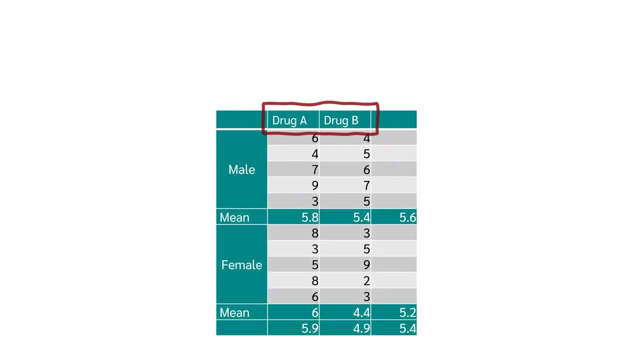 and it all adds up in the error. But how do we calculate the sum of squares, the F-value and the P-value? Here we have our data, once drug type, with drug A and B, and once gender, with male and female. So these individuals are, for example, all male and have been given drug A. 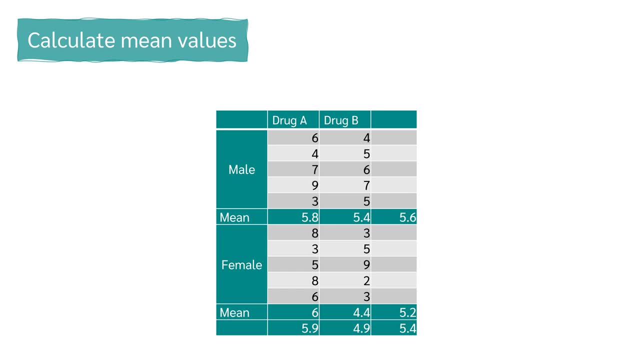 First we calculate the mean values for drug A and B. We calculate the mean value of each group, so male and drug A, that is 5.8, then male and drug B, that is 5.4. and we do the same for female. 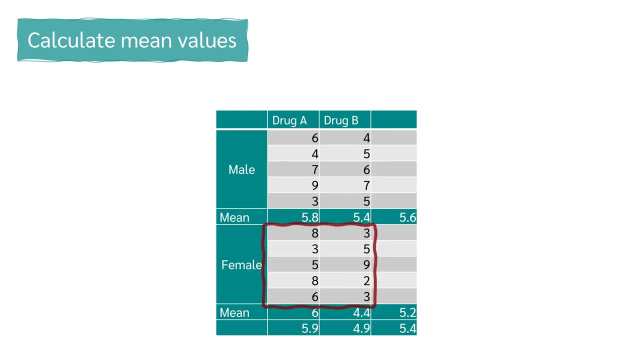 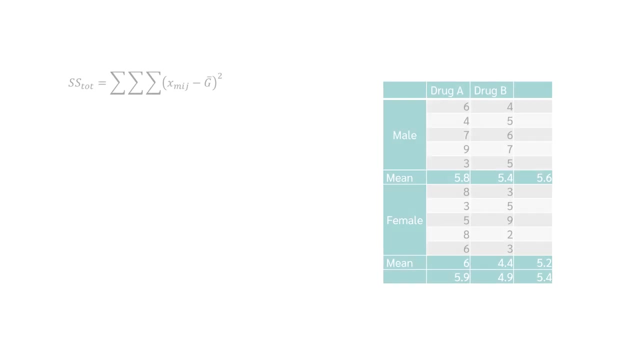 Then we calculate the mean value of all males and females and the mean value of drug A and B. Finally, we need the total mean. We can now start to calculate the sum of squares. Let's start with the total sum of squares. We do this by subtracting the total mean from each individual value, squaring the result. 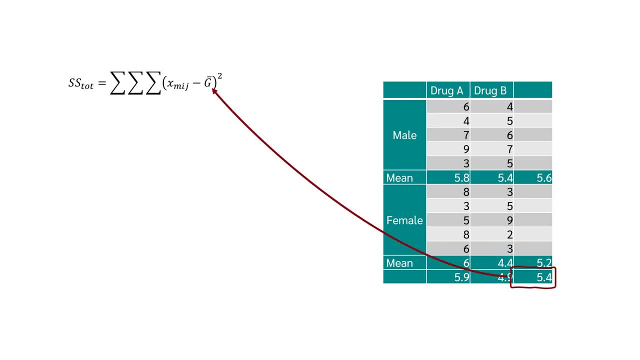 and adding up all the values, The total mean is 5.4, so we calculate 6 minus 5.4 squared plus 4 minus 5.4 squared to finally 3 minus 5.4 squared, So we get a sum of squares of 8.4.. 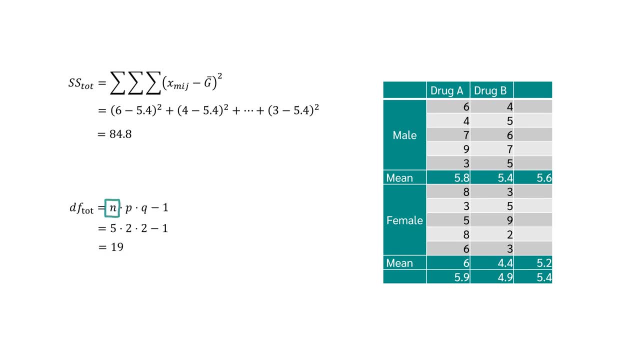 84.8.. The degrees of freedom are given by n times p times q minus 1.. n is the number of people in a group, in our case 5, and p and q are the number of categories in each of the factors. 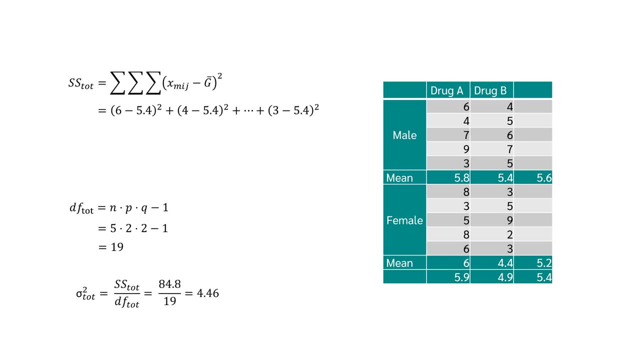 In both cases we have two groups. The total variance is calculated by dividing the sum of squares by the degrees of freedom. So we get 4.46.. Now we can calculate the sum of squares between the groups. For this we calculate the group mean minus the total mean. 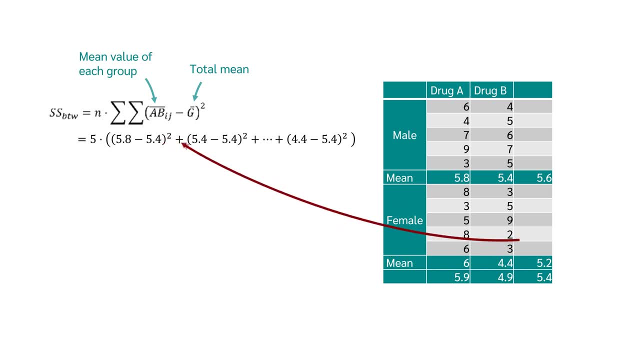 So 5.8 minus 5.4 squared plus 5.4 minus 5.4 squared and the same for these two values, We get 7.6.. In this case, the degrees of freedom are 3, which gives us a variance of 2.53.. 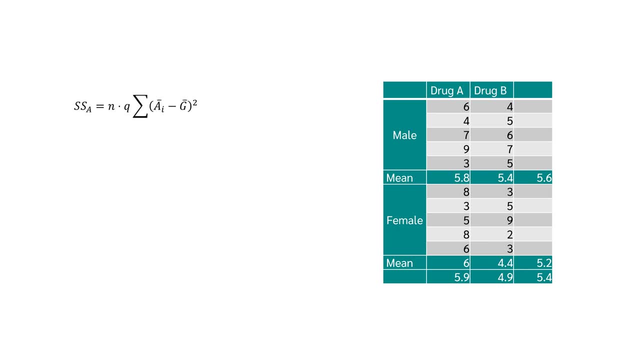 So we get 7.6.. So we get 7.6.. Now we can calculate the sum of squares of factor a. a dash is the mean value of the categories of factor a. So we calculate 5.9 minus the total mean value and 4.9 minus the total mean value. 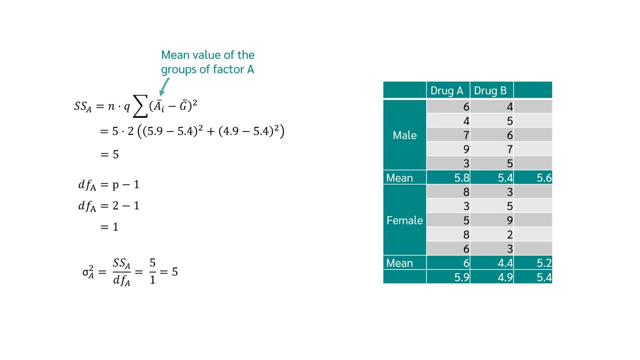 This results in 5.. Together with the degrees of freedom, we can now calculate the variance for factor a, which is 5.. We do the same for factor b. In this case, we use the mean. We use the mean values of male and female. 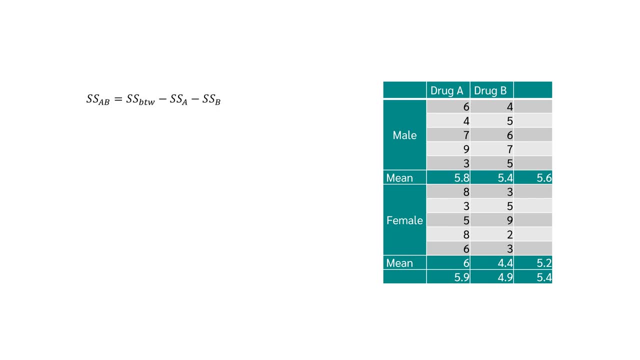 And we get the variance of 0.8.. Now we can calculate the sum of squares for the interaction. We obtain this by calculating the sum of squares minus the sum of squares of a and b. The degrees of freedom result to 1.. 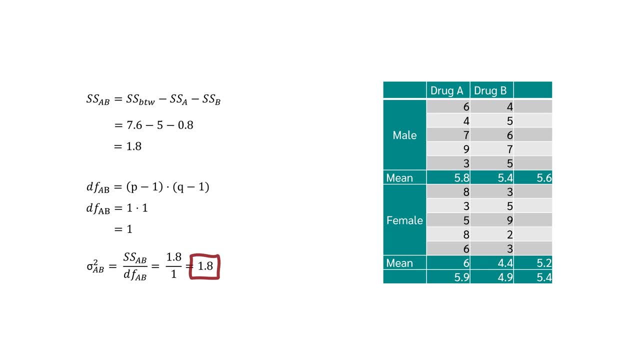 For the interaction. we get the variance of 1.8.. Finally, we can calculate the sum of squares of the error. We subtract the mean. We subtract the mean value of each group from the respective group values. So in this group we subtract 5.8 from each individual value.